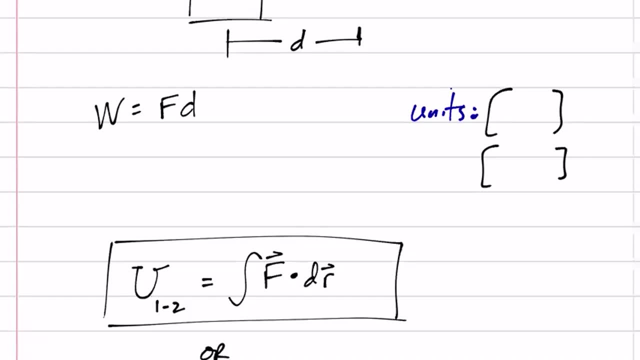 And what about that dot product? You know how a dot product works. You take the x component times the x component. plus, you take the y component times the y component. you take the- You know z component times, the z component. Right now I'm on dot product. But does that kind of make sense? if you want the force? 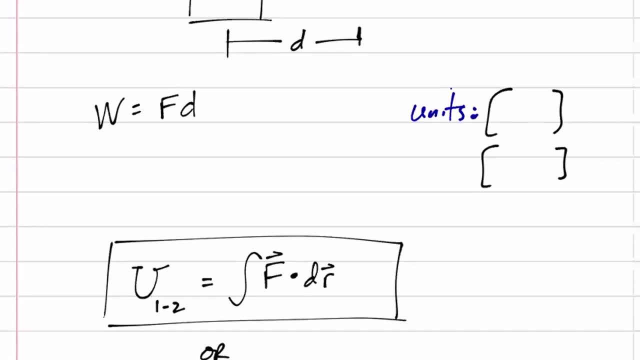 only in the direction. It's kind of like taking the x component of force times the x displacement Plus maybe the y component of force times the y displacement, The z component of force times the z displacement and then adding those up And that's a total work done. 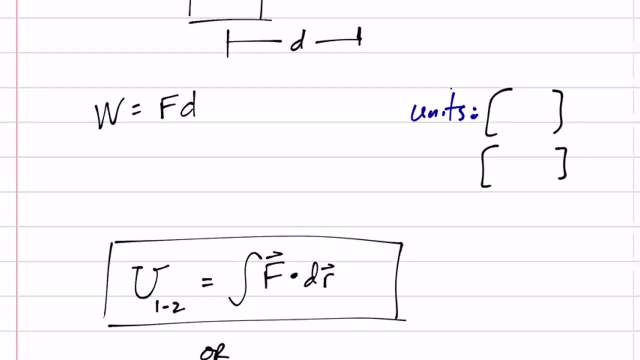 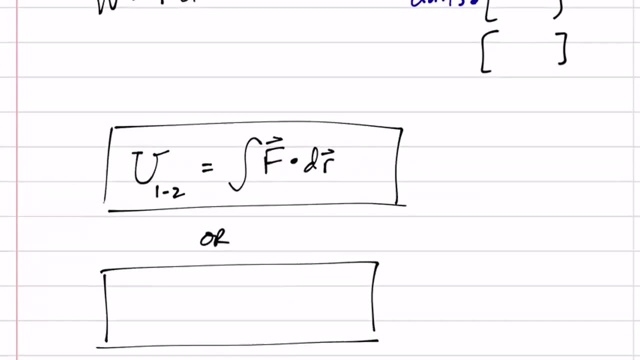 Kind of like the work done by the x force in the x direction work done. When you add those up, when you dot product two vectors, you only get a scalar. You don't end with a vector. So this is just a scaler. 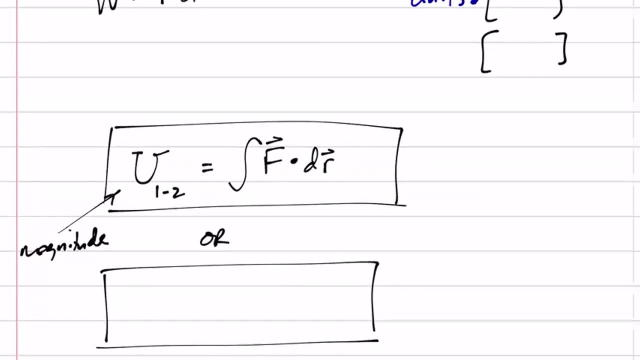 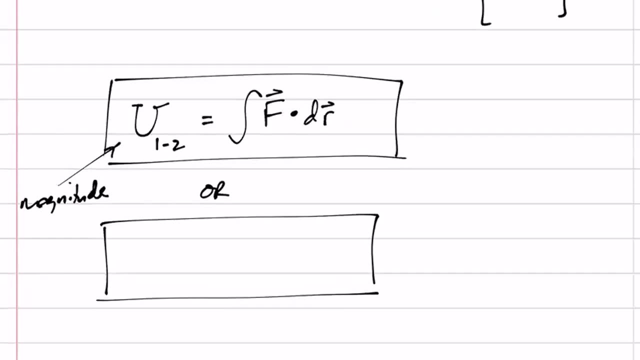 This is the magnitude, The magnitude of work would be. if we could, we would integrate our force vector, dotted with our differential position vector, from one to two, Or maybe another way of thinking about this, the work done from one to two. 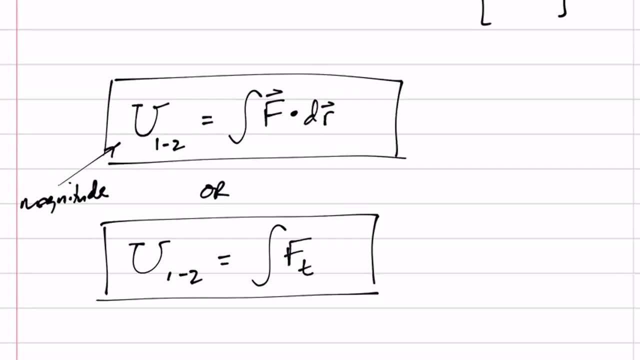 What if we only consider this��터 tangential component of force, ds. so if we're only worried about the tangential component of force, if we're only worried about the component of force that is actually in the direction, then we could integrate F tangential times, ds. So if we 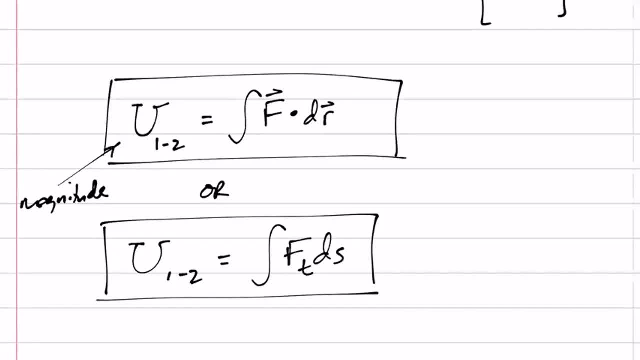 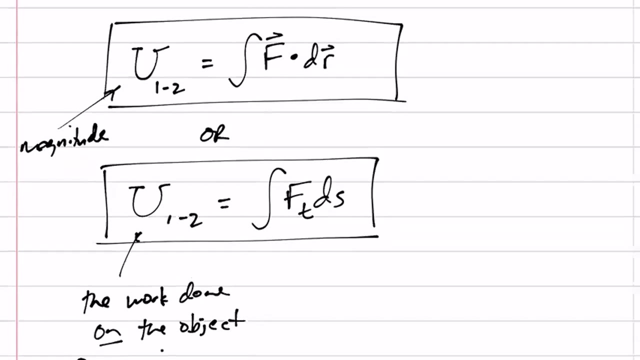 want to write this in words. it would be the work done. let's actually write this, the work done on the object from position one to position two, All right, and it would be equal to the integral of F tangential. if we had an equation for F tangential, or maybe. 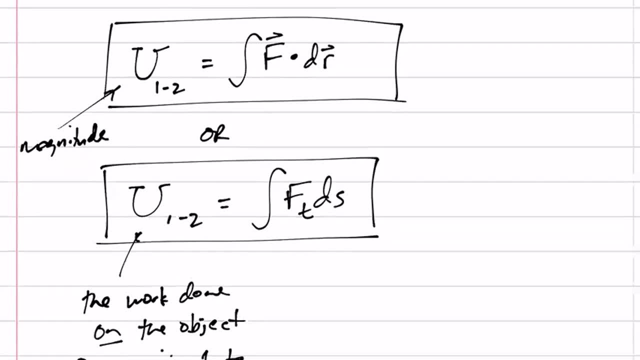 if we're lucky, F tangential is just constant. Right, But if it's not constant, we would have to integrate it with respect to S, And F tangential would be the force that's in the direction of the displacement. All right, 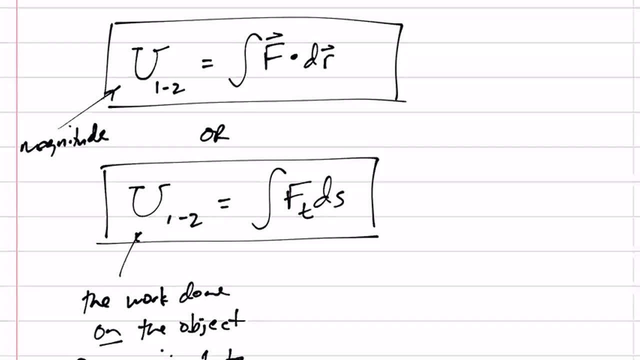 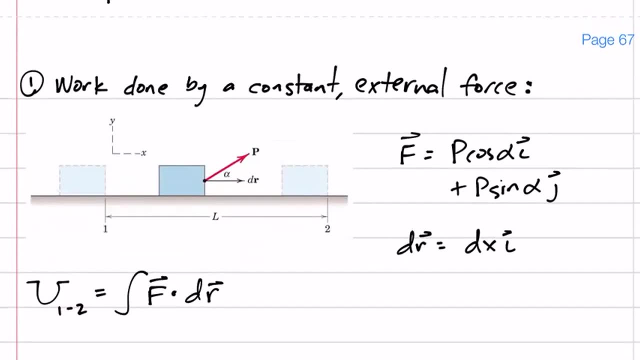 But I'm not going to want to do these integrals every time. Let's look at some common scenarios, Let's go ahead and do the integral And let's get an equation for the work for common things that we'll see Okay. 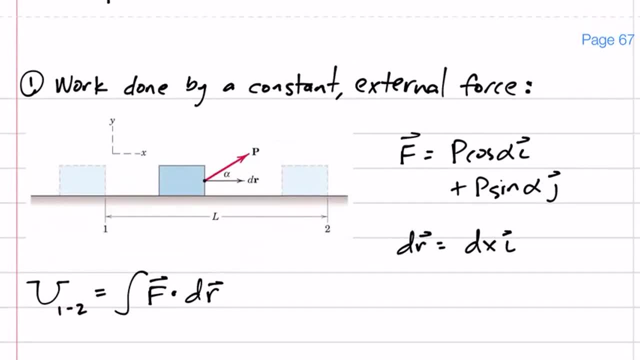 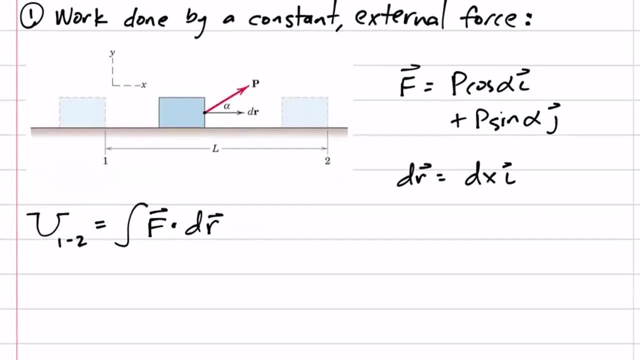 This page and the next page I will print out for you. I'll post them, I'll print out, I'll bring them to class. But if we were looking at a constant force F, so maybe don't write this down or just kind of sit back and listen. 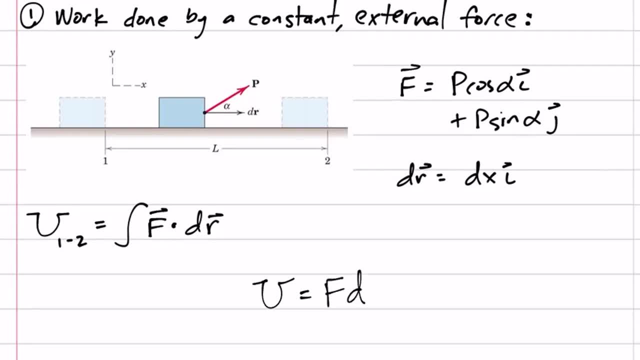 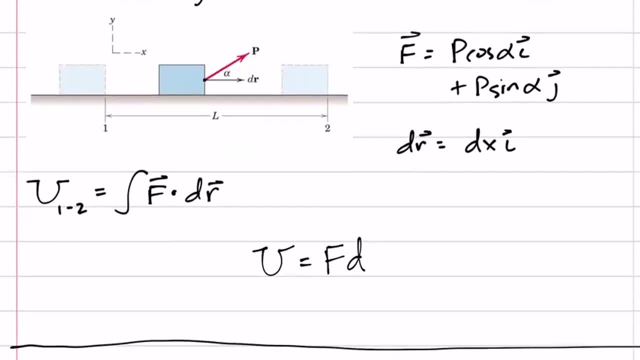 Work is force times distance, but it's only the force that's in the direction of the distance. So in this case, if it's a constant force, we kind of bring it out of the integral. The U would be P, cosine, alpha times L. 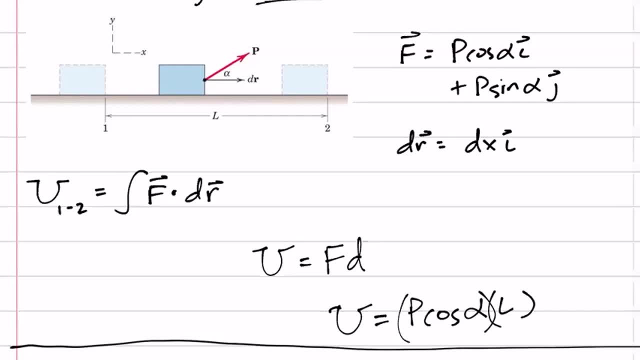 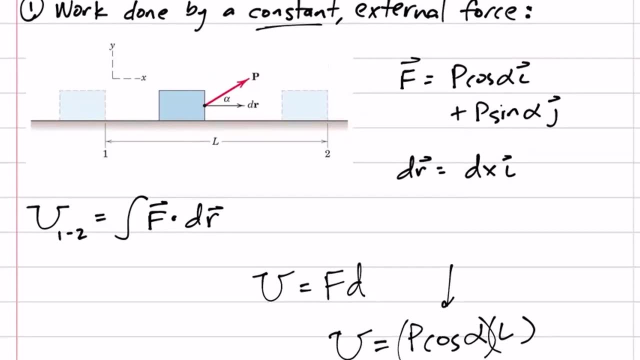 Does that make sense? Makes sense that this, in this case, for a constant force? you would just take the component of force that is in the direction of the distance times the distance. All right, Just take the component of force in the direction of the distance times the distance. 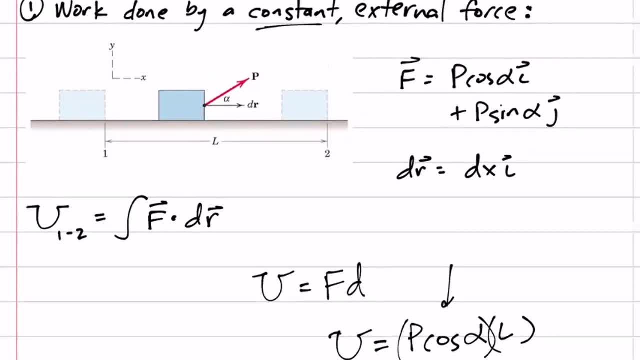 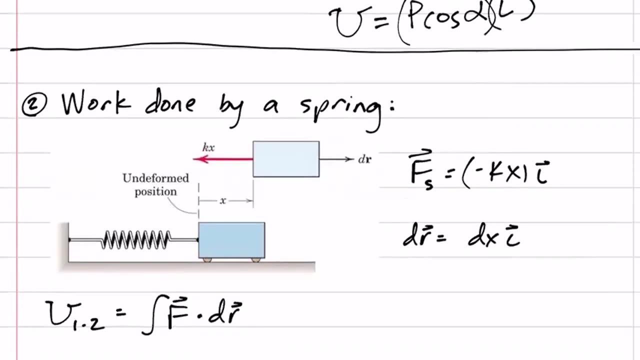 Now, it's not always going to be cosine, You know. just look at the setup, Look at what angle you need to find only the component that's in the direction of the displacement. Okay, How about work done by a spring? If we were to integrate this with respect to X, it might be something like an X squared over two. 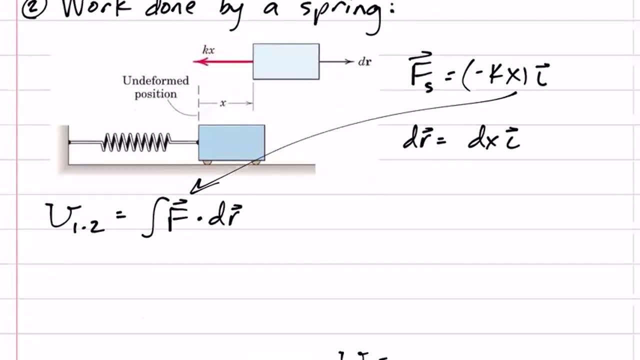 All right, You can look at this, but it would be, the work done by a spring would be one half K X, one squared minus X, two squared. All right, And so we can use that equation if we want to know the work, If we want to know the work done by a spring. so we don't have to say, well, the force is K X. 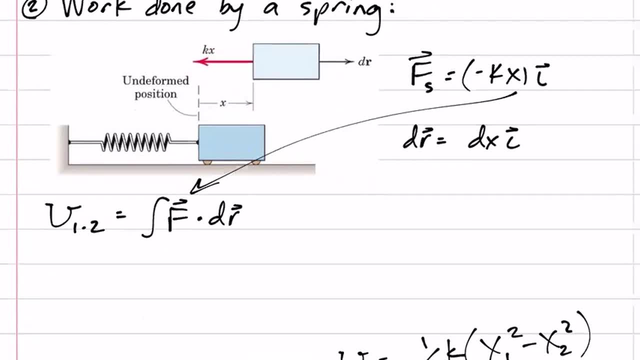 I need to integrate. You can just say: hey, the work done by spring is one half K X one squared minus X two squared. Be careful That X one is not the length of the spring. It's the amount of stretch or compression of the spring. 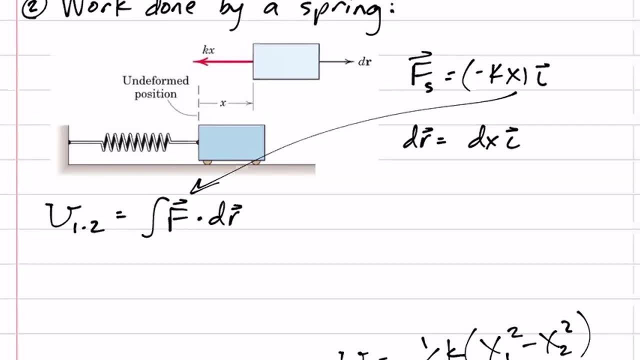 So technically we might put delta X squared minus delta X squared. Those X's are stretches or compression. All right, And also be careful, It's easy to kind of get these backwards. We are calculating the work done on an object And so we've got X initial squared minus X final squared. 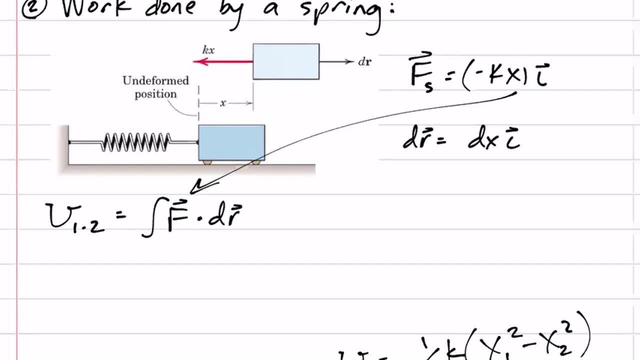 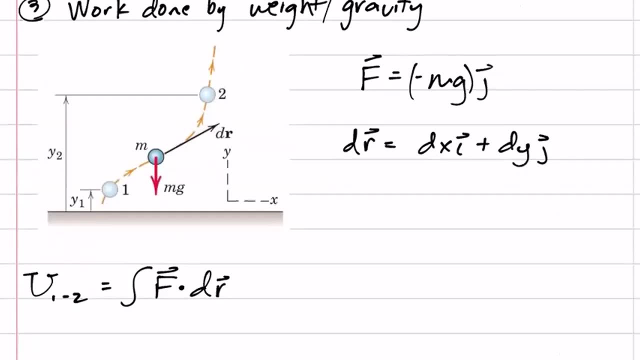 But anyway, so we can use that equation if we want to find the work done by a spring, If we want to find the work done by gravity, Now hold on till next class, because I don't really like thinking about gravity as done by gravity. 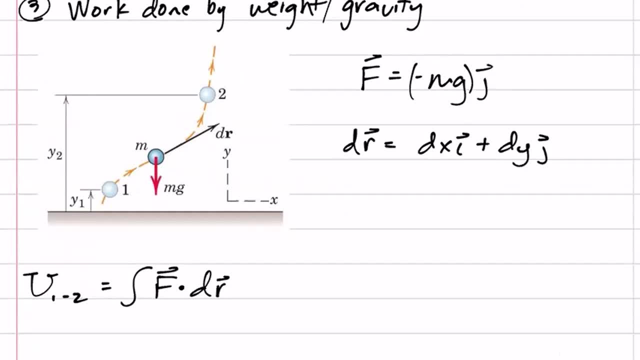 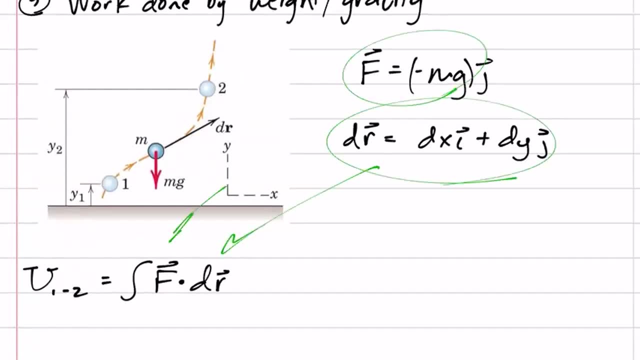 I don't like doing work. Next class we'll talk about potential energy for gravity and for a spring. But we could. we could plug this in right here. We could do the integral. You know we would get the work done is M G. 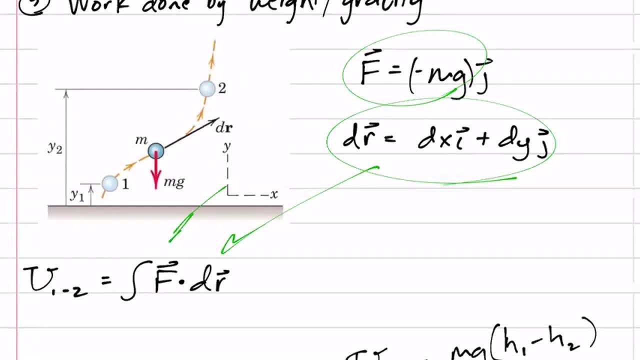 I like to write these as H one minus H two. The book might say Y one minus Y two, But H is the vertical position And, be careful, It's one Minus two. So anyway, if we want to know the work done by gravity, then we've got an equation. 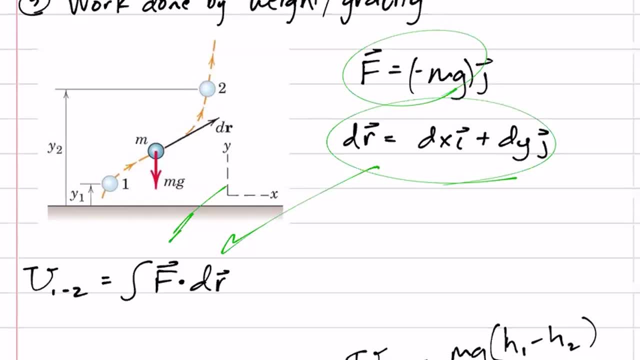 M, G, H one minus H two. We don't have to do this integral, We just did it. I'll give it to you in your notes. We did the integral. We can just use this, That equation, to find the work done by gravity. 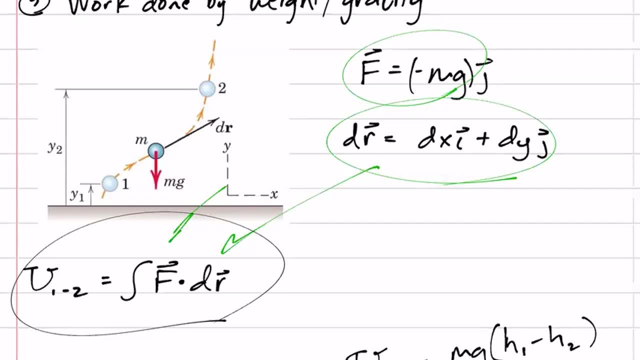 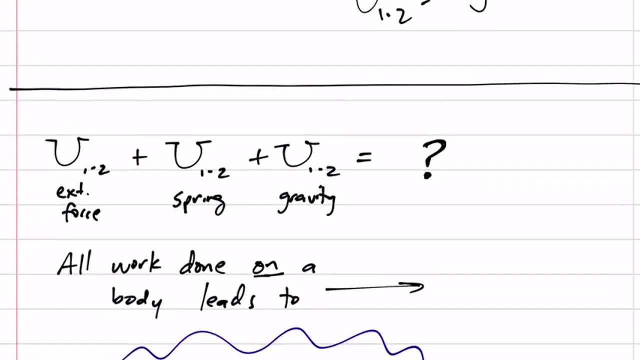 All that it depends on is where its initial height was and where its final height is Doesn't matter. It doesn't matter if it came somewhere and came back its initial and final, All right. But why would we use these? We can add up all the work done by forces plus the work done by spring, plus the work done by gravity. 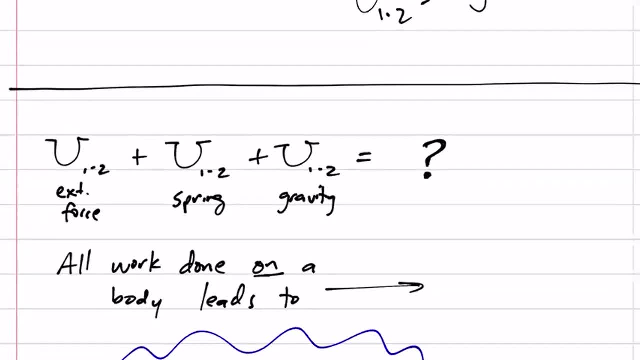 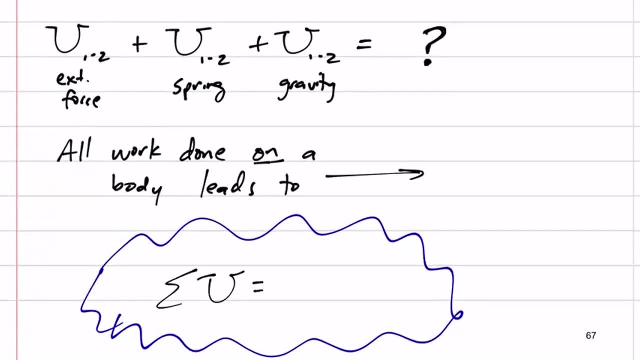 And it all would lead to the right hand side. What do you think the right hand side of this equation might be? That's right. Sum of all the work equals something I don't know if you already know. I don't know, if you already know. 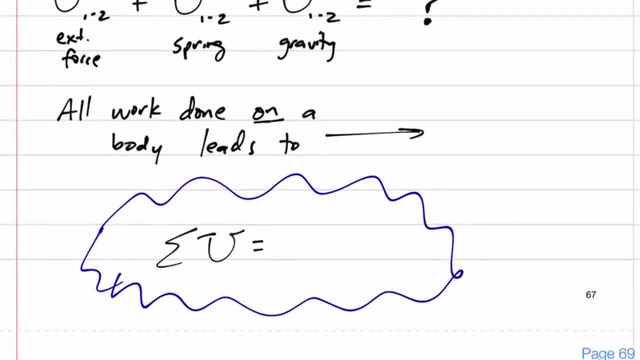 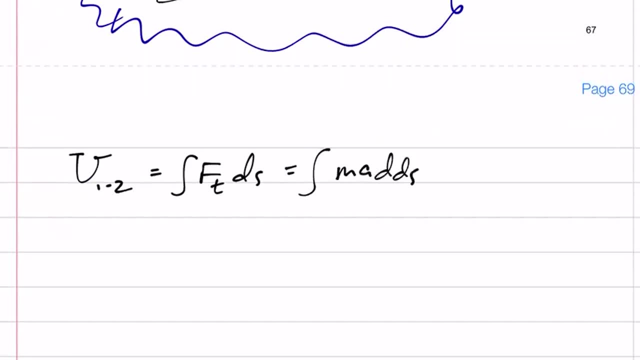 Real quickly on the left hand side, if we substituted M A, if we substituted M A for force, and we'd end up with the integral of A D S, what is the integral of A D S, V D V, V And what is the integral of V D V? 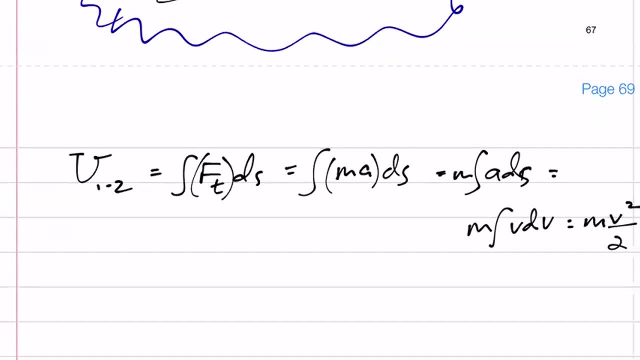 V squared over two, But this is a definite integral. What we would end up with is one half M V two squared. one half M V- one squared. What is one half M V squared? Kinetic energy. Kinetic energy. Kinetic energy. 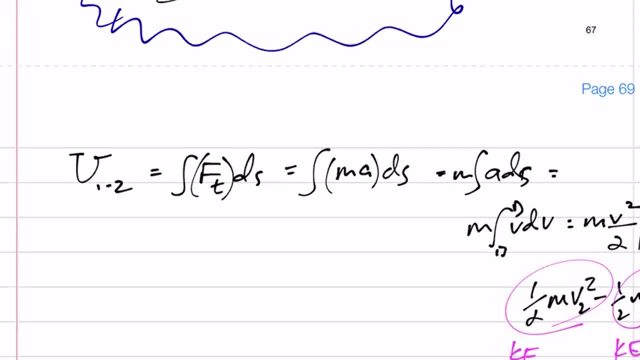 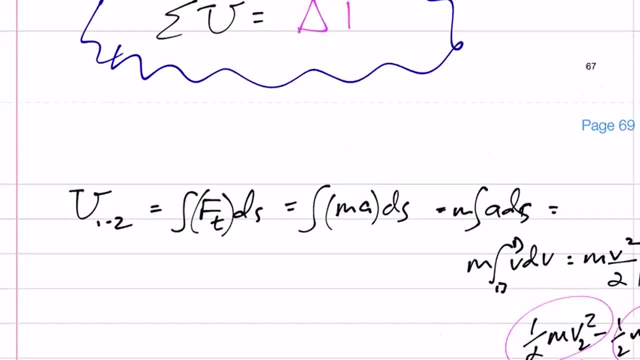 The sum of all the work leads to the change in Kinetic energy. Instead of K? E, we're going to write this as capital T. So here we go. The sum of all work equals the change in kinetic energy. Maybe you could write that in words. 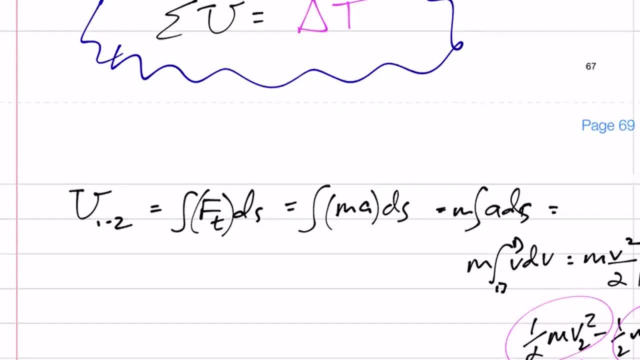 The sum of all the work done equals the change in kinetic energy. So we're going to say: okay, left hand side of my equation: What is the work done by gravity: M, G, H, one minus, H, two plus? what's the work done by spring? 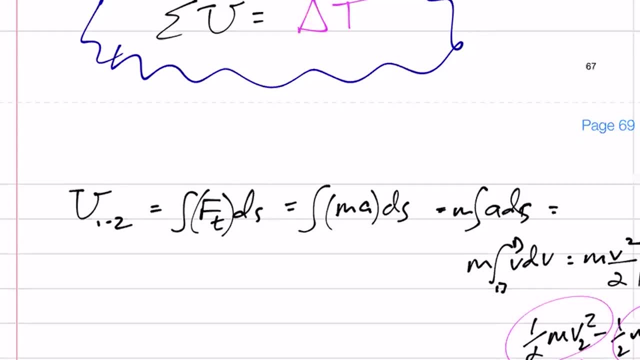 Plus what's the work done By this force? That's the left hand side of my equation. The right hand side of my equation equals one half M V, two squared, minus one half M V, one squared. Okay, So I'll maybe fill this out. 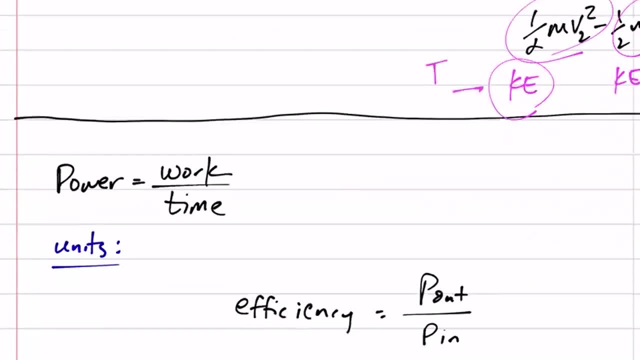 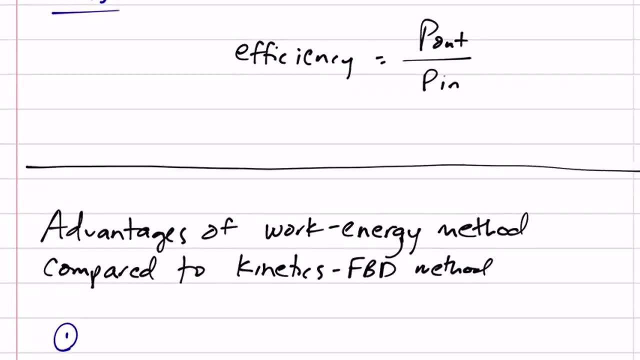 Power is work over time, Efficiency is out over in. But last thing, I want to mention two minutes. This is a new method. How is this different from what we have been doing? We have been drawing free body diagrams and some of the forces is mass times, acceleration. 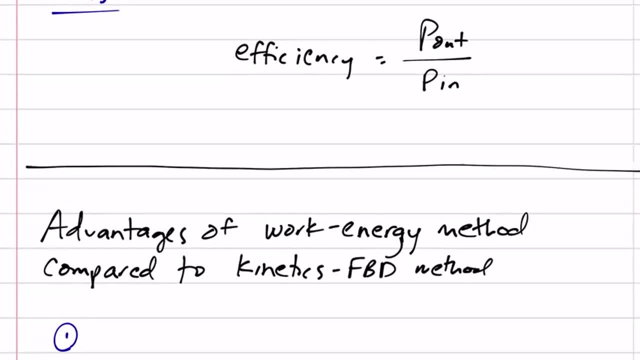 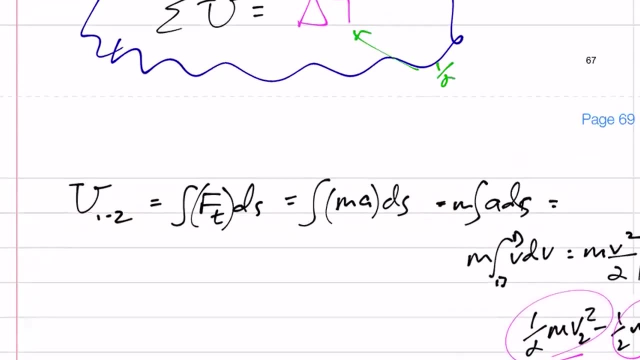 Now we're going to be looking at work and energy. the main difference, The main difference, is One half M, V, V, V, V. these equations will lead us straight to velocity, Our other problems. we had to have been doing. we had to sum the forces.